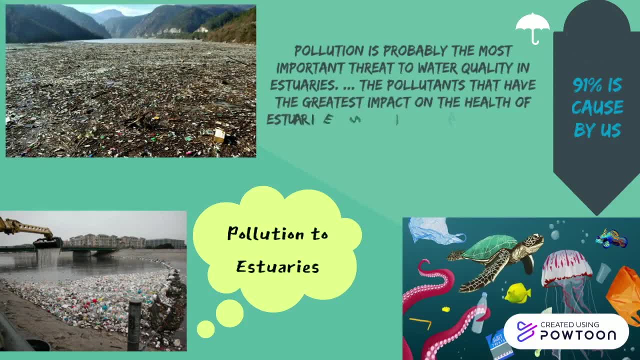 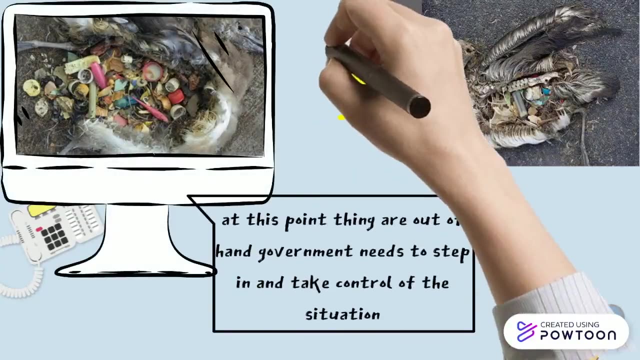 The pollutants that have greatest impacts on the health of the estuaries include toxic substances like chemicals, heavy metals and nutrients. pollution and pathogens such as bacteria and viruses also cause damage to the estuaries. Eutrophication is often devastating to animals. 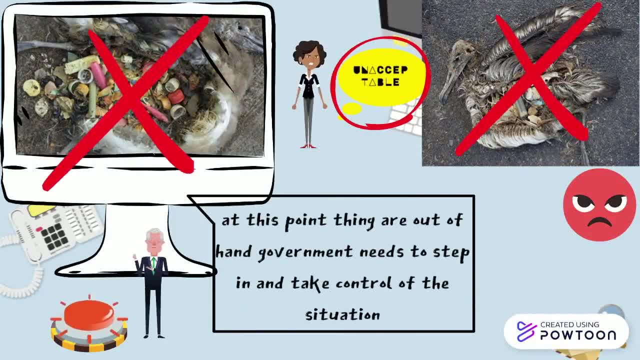 and plants in estuaries, as well as economics of communities surrounding estuaries. Toxic algal blooms disrupt tourism due to poll orders and unsightly views. At this point, things are out of hand and the government needs to step in and take control of. 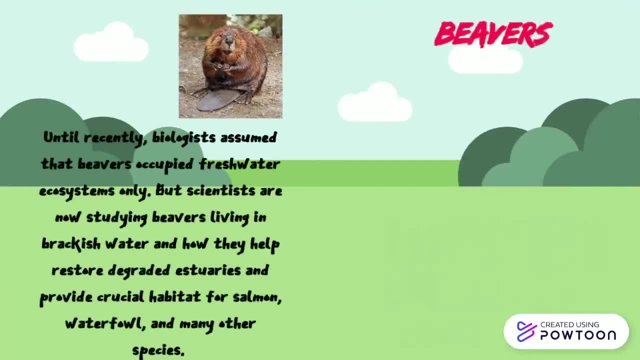 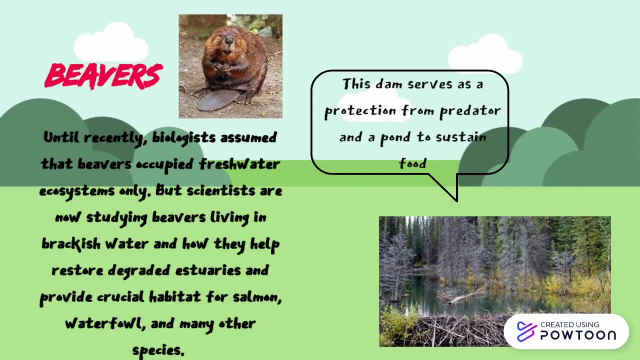 this situation. Beavers are fascinating creatures that play an important role in establishing and maintaining wetlands. Learning to live peacefully with these animals is important to the health of their environment. Beavers' dams enhance their environment by providing habitats for many sensitive plants and animal species. Until recently, biologists assumed that beavers 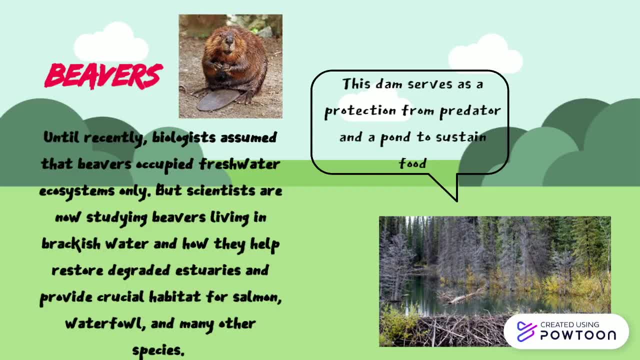 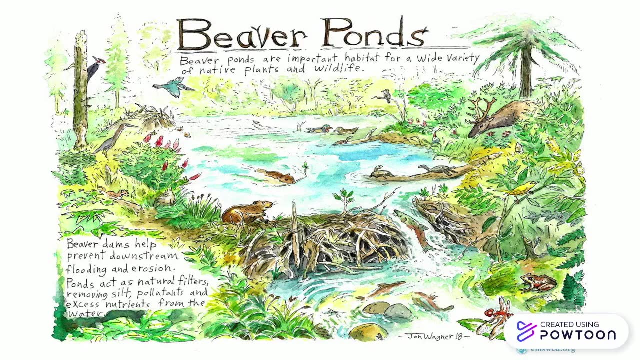 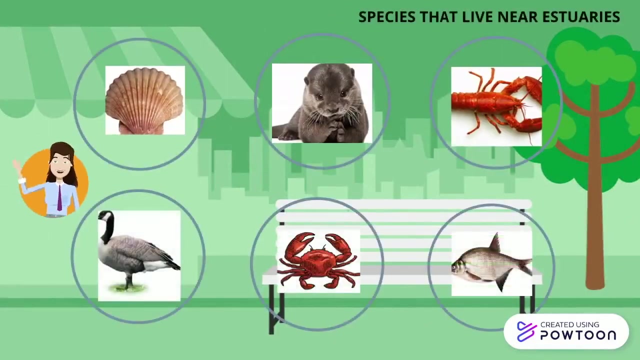 occupy freshwater ecosystems only, But scientists are now studying beavers living in brackish water and how they help restore degraded estuaries and provide crucial habitats for salmon, waterfowl and many other species. Several types of different species can be found in estuaries. 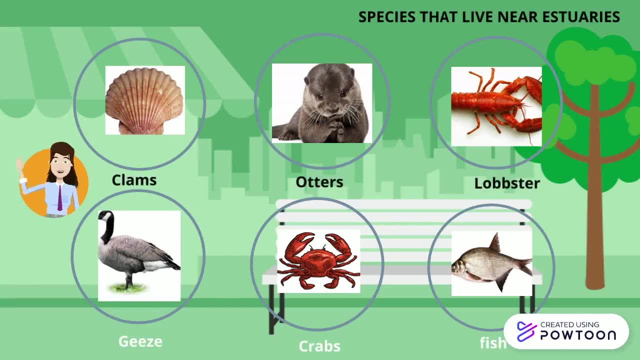 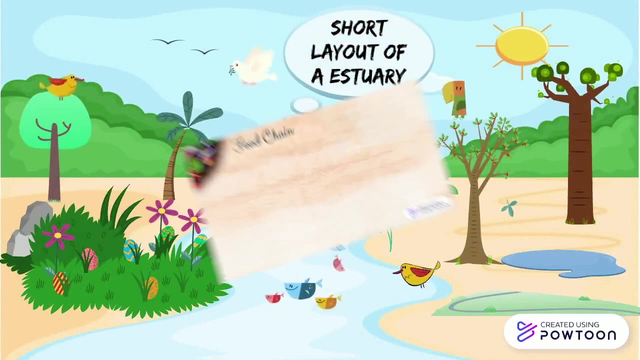 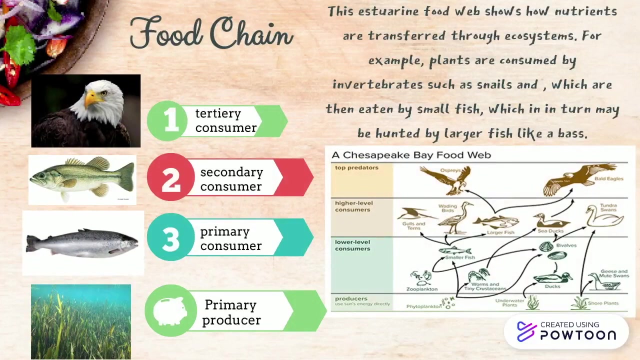 but the most common ones are clams, otters, lobsters, geese, crabs and different types of fishes. Food chains: This estuarine food chain web shows how nutrients are transferred to the estuaries. For example, plants are consumed by invertebrates, such as snails, which are then eaten by small. 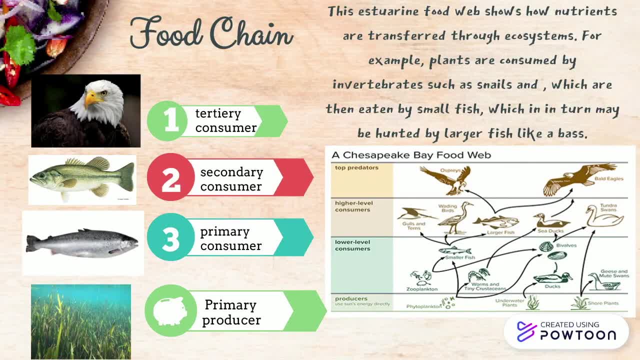 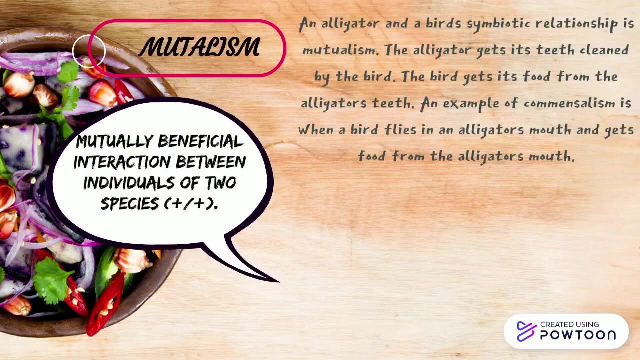 fishes, which is then turned into, or may be hunted by larger fishes like bass, which is then hunted by tertiary consumers, known as the bald eagle. Mutilism is a mutually beneficial interaction between individuals of two species. An alligator and a bird simply have a similar